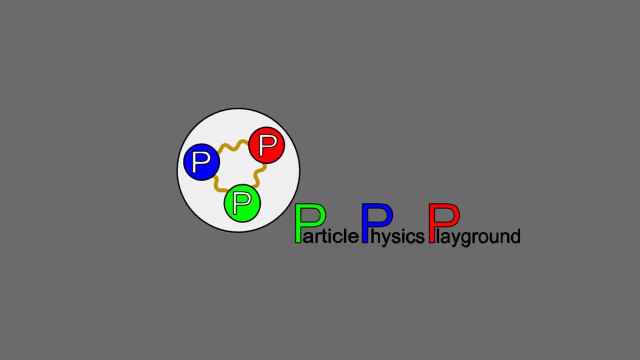 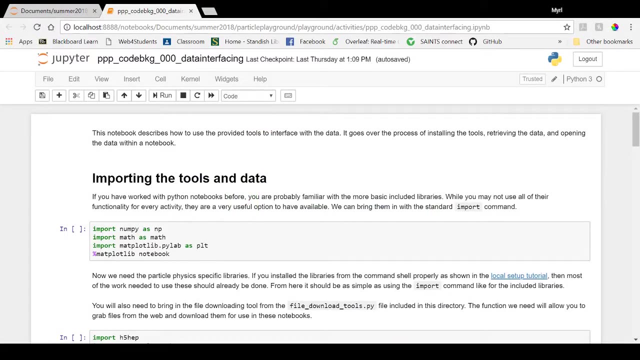 This is a brief summary on how to import the tools for running Particle Physics Playground on a local Python notebook installation. We will be going over the documentation in the first part of the Data Interfacing Notebook. First we can import the standard Math NumPy. 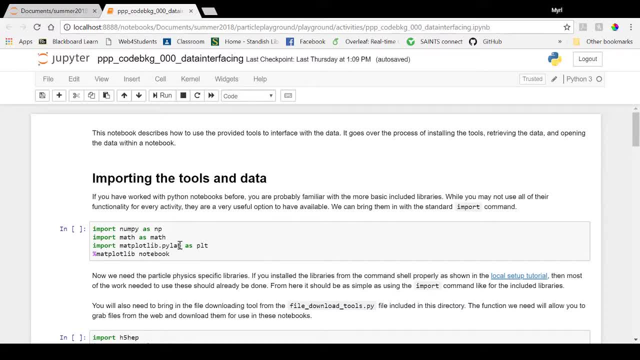 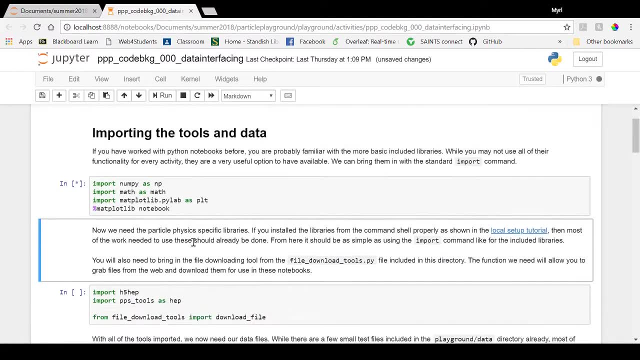 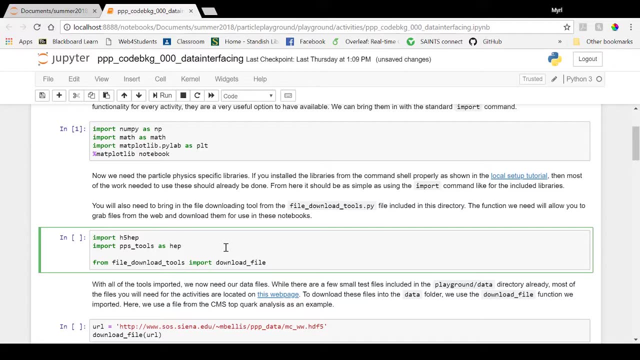 and PyLab libraries, like usual, using the import command. Remember to include the %matplotlib with notebook or inline commands to be able to see the output of your plots. Now, if you properly installed the H5HEP and Particle Physics Simplified libraries, as shown, 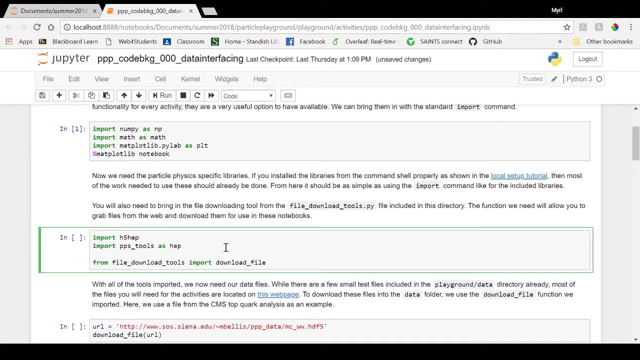 in the Local Setup video tutorial. using these tools should be as simple as importing them as you would with the local libraries. You will also need to import the download file function from a file within the activities folder itself. This is also done with the import command. 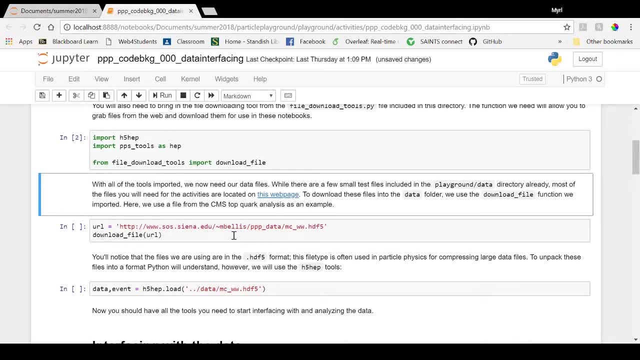 The download file function you imported allows you to download files from the web, which is necessary because most of the files you need for the activities in Particle Physics Playground are located on this website, which is also linked in every activities notebook. Simply change the URL to whichever file you need and run the command. It will download. 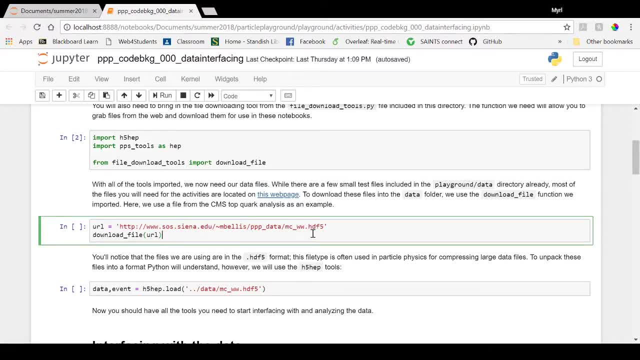 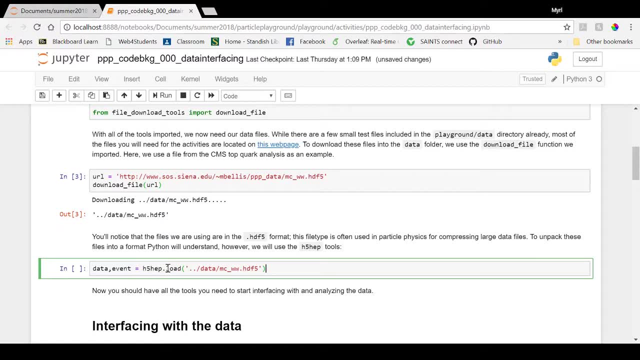 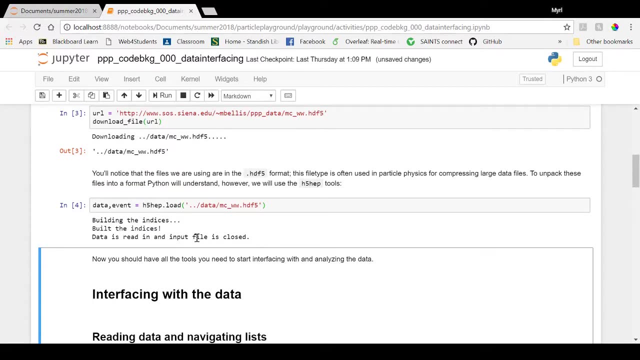 the data directly into the data directory within the main Playground folder. You can then use the H5HEP tool's load function to be able to unpack the data from that location. Those are all the tools you will need to import, to download and interact with the data in. 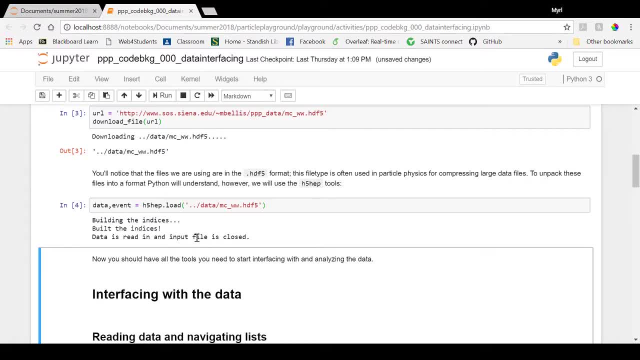 all of the Particle Physics Playground activities You can get started now or, for more background, you can check out the video on how to interface with the data, which covers the content discussed in the second half of this notebook.